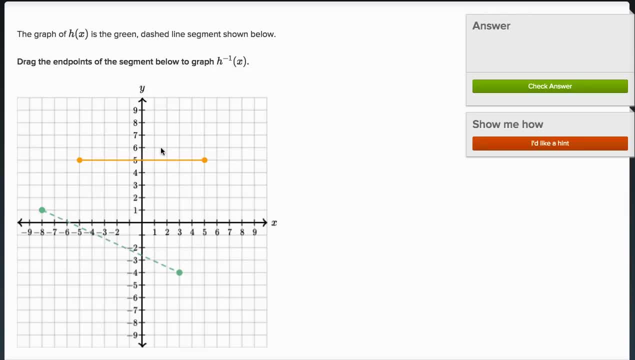 This right over here is our understanding inverses of functions exercise on Khan Academy And it's a good exercise to make sure you understand inverses of functions. And it's an interactive one where we can move this line around And they tell us the graph of h, of x is in green. 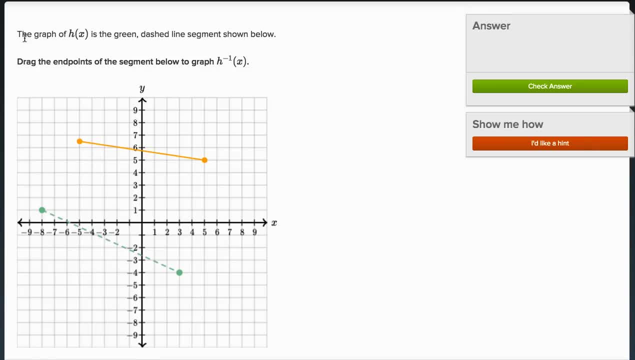 So that's this dotted green line right over here. The graph of h of x is the green dashed line segment shown below. so that's this: Drag the endpoints of the segment below to graph h, inverse of x. So there's a couple of ways to tackle it. 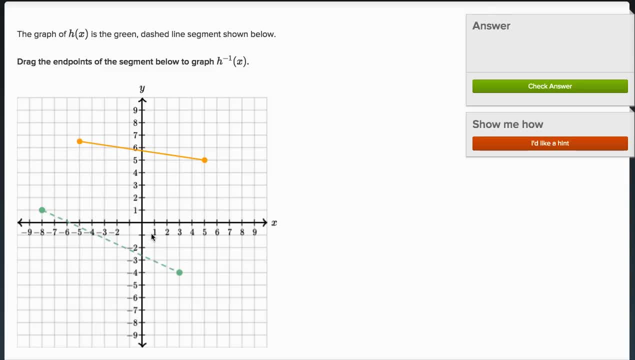 Perhaps the simplest one is we say: okay, look, h of x. what does h of x map from and to? So h of x. this point shows that h of x. if you input negative eight into h of x, h of negative eight is one. 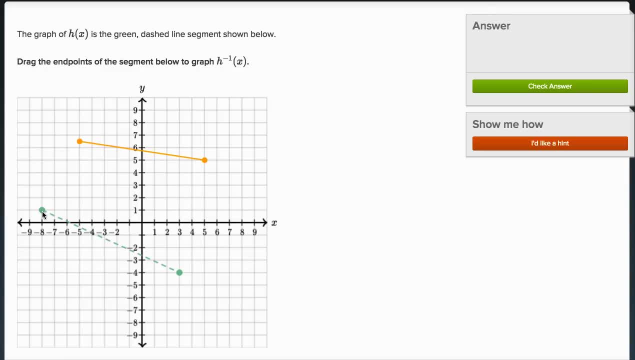 So it's mapping from negative eight to one. Well, the inverse of that, then, should map from one to negative eight. It should map from one to negative eight. So let's put that point on the graph of the inverse And then let's go on the other end. 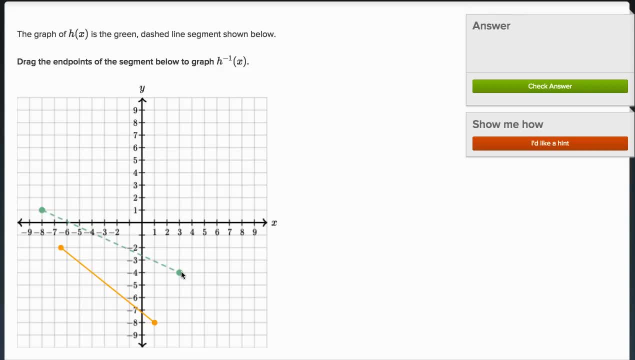 So let me just move this a little bit out of the way. On the other end of h of x, we see that when you input three into h of x, when x is equal to three, h of x is equal to negative four. 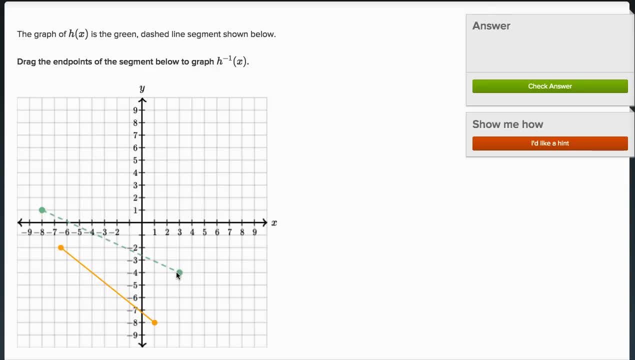 So this point shows us that it's mapping from three to negative four. So the inverse of that would map from negative four to three. So if you input negative four, it should output three. If you input negative four, it should output three. 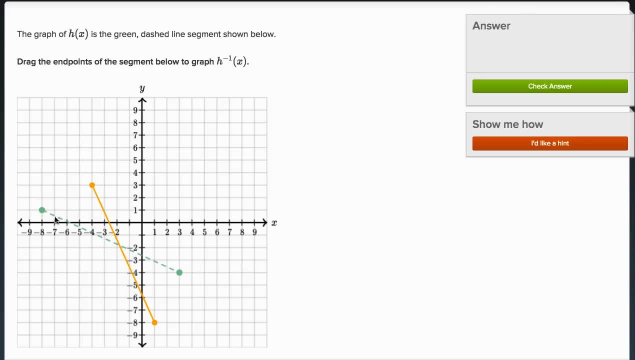 And since we took the two points and we took the two endpoints of this line and we essentially found the inverse mapping of it, what I've just done here is I've graphed the inverse. And another way to think about the inverse is if you were to draw the line, y equals x. 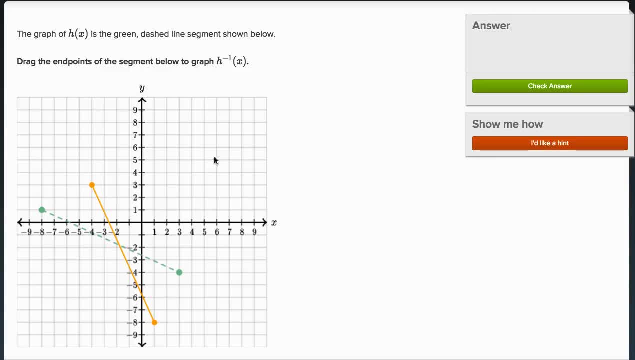 So I don't have my little pen tool right here because I'm operating on a webpage, But if you imagine the line y equals x, these things should be reflections around the line y equals x, Because one way to think about it is you're swapping. 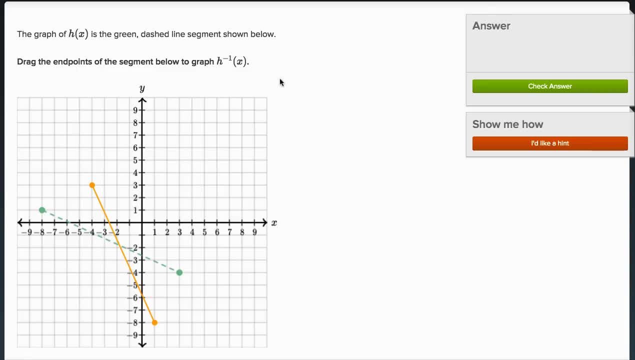 the x's for the y's over here. And you see that If you were to draw the line y equals x, these things, if you flipped it around, the line y equals x, the green line, you would actually get the yellow line.